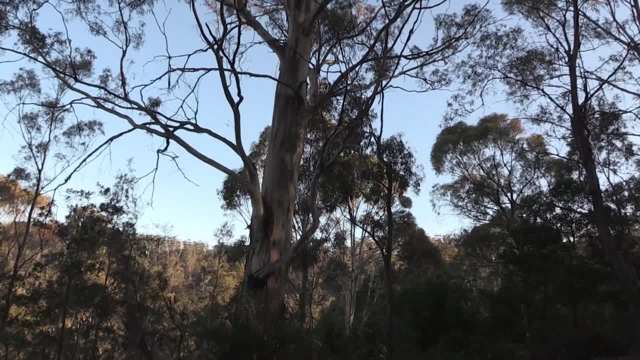 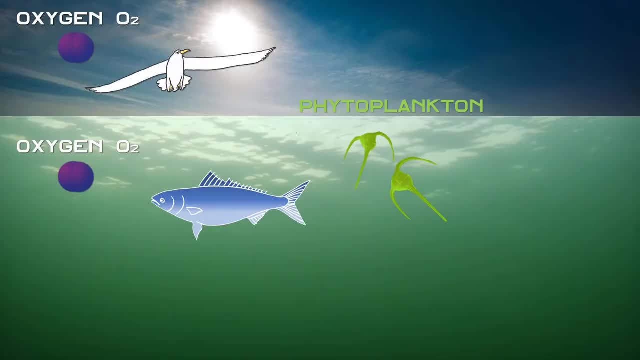 disturbed, as in this sample in a bucket demonstrates. Like plants on land, phytoplankton in the sea breathe. In order to survive, animals need oxygen, which they can obtain by breathing from the air or from the water, where it can be dissolved. The animals will use the oxygen, which is then converted into carbon dioxide, which 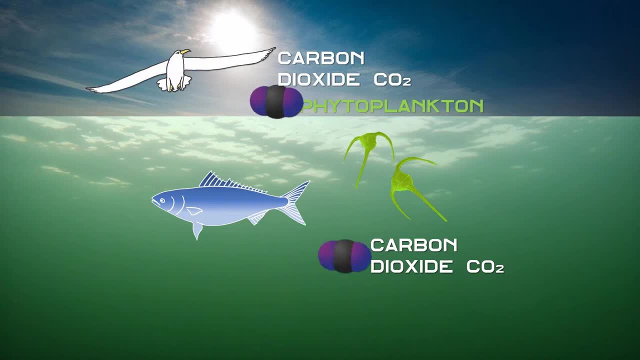 they then breathe out. The carbon dioxide in the air can also dissolve into water. Plants, including phytoplankton, need carbon dioxide to survive, so they breathe it in. They use the carbon dioxide, then breathe out oxygen, which can then also be released into the air. At least half of the oxygen in the atmosphere has come. 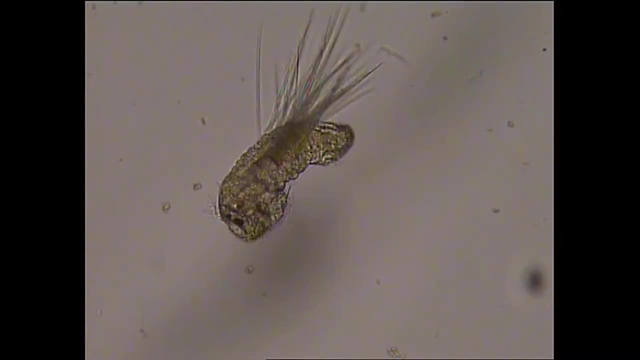 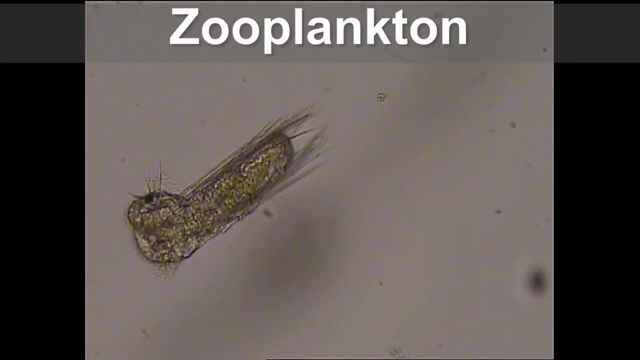 from these microscopic phytoplankton in the ocean. As mentioned earlier, the other main group of plankton are animals, and they are called zooplankton. Within the zooplankton, there are two main types: Those that spend their entire life cycle as 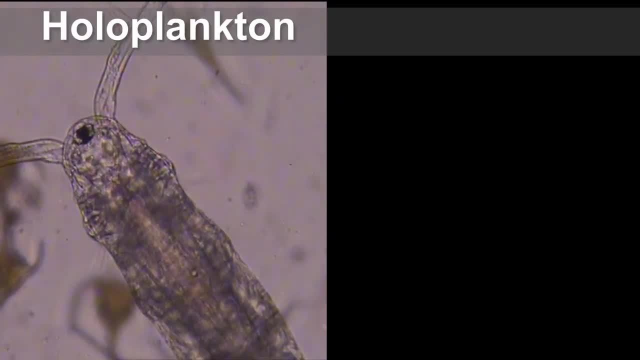 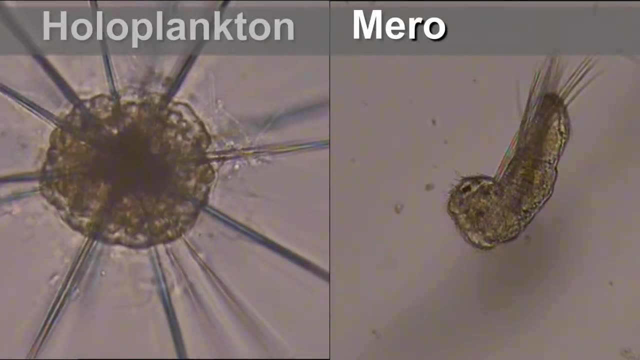 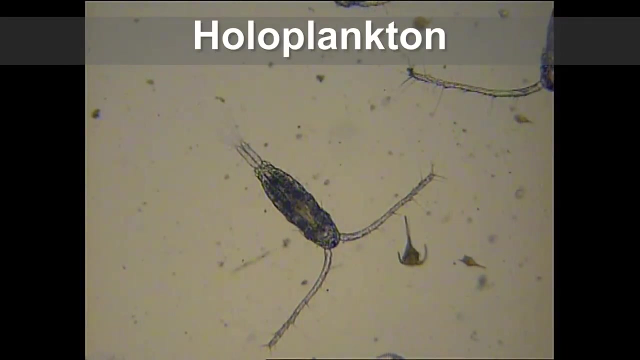 microscopic plankton and we call these holoplankton and the other type that are just babies of much larger animals that are beginning the first stages of their life cycle and we call these meroplankton. Examples of holoplankton that you will see under the microscope include 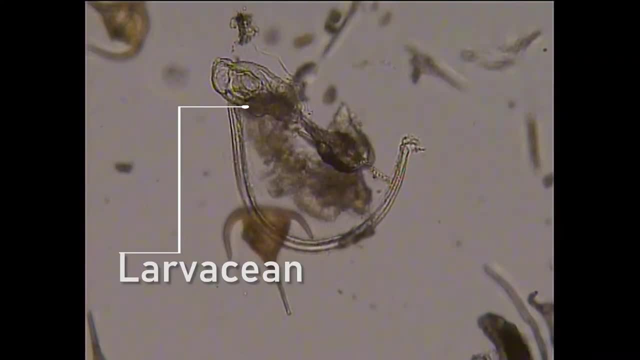 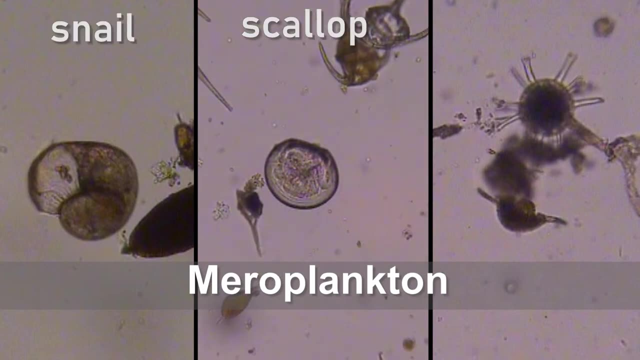 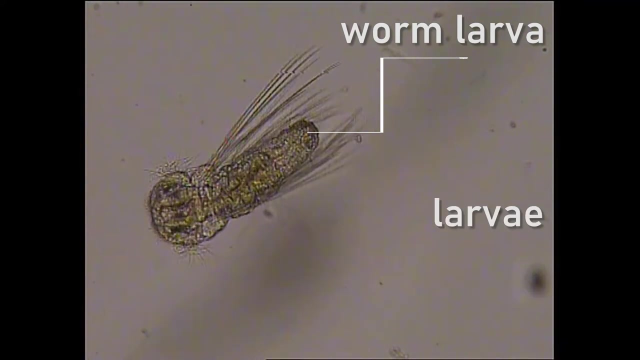 copepods and larvaceans. Examples of meroplankton that you might find include baby snails, scallops and sea urchins. When a zooplankton is a baby, we call it a larva, The plural is pronounced larvae. Sometimes you might find a circular. 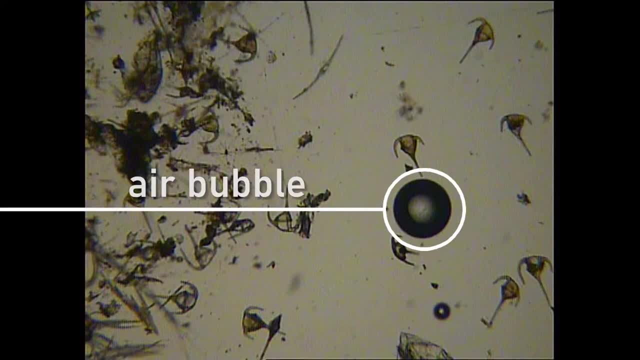 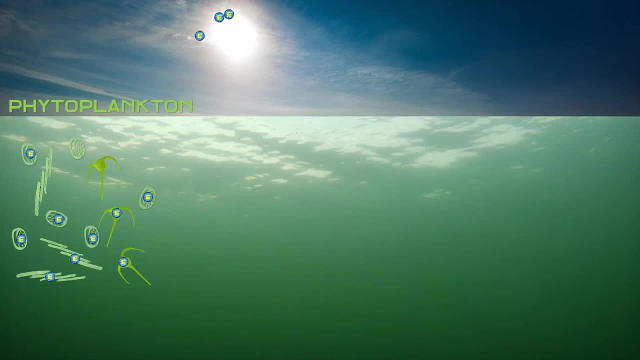 thing with a very thick black outline. This is an air bubble in your sample, not a plankton. The tiny phytoplankton absorb energy from the Sun and knock it in their body. as chemicals, This is a vital food source for the zooplankton. When zooplankton eat them, they take up the phytoplankton's energy. 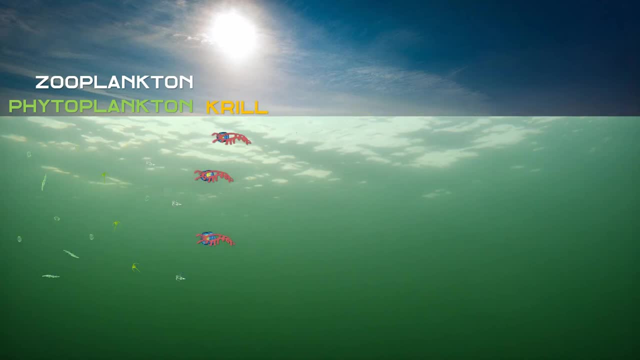 Other animals, such as krill, eat the zooplankton and the phytoplankton, which in turn, are eaten by other animals such as fish, and we can see how the energy moves through the food chain. At the Marine Discovery Center, we collect our plankton each morning from